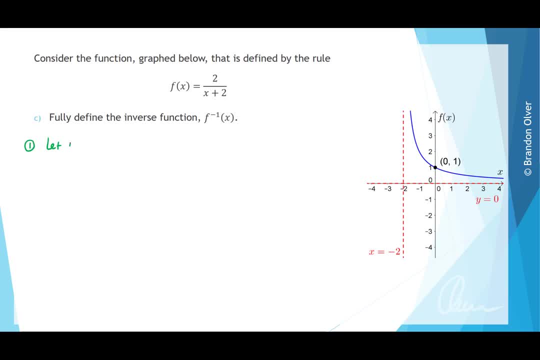 So the first thing we're going to do is let y equal f of x. So this gives us: y is equal to 2 divided by x plus 2.. And the second step is to swap x and y To find the inverse function. 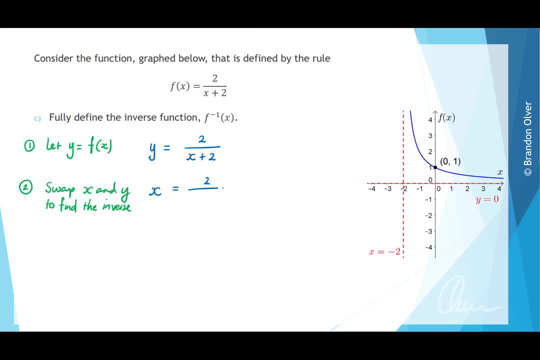 So that will give us: x is equal to 2 divided by y plus 2.. Step 3 is to solve for y. So to do that, we're going to start by multiplying by y plus 2.. For both sides of the equation. 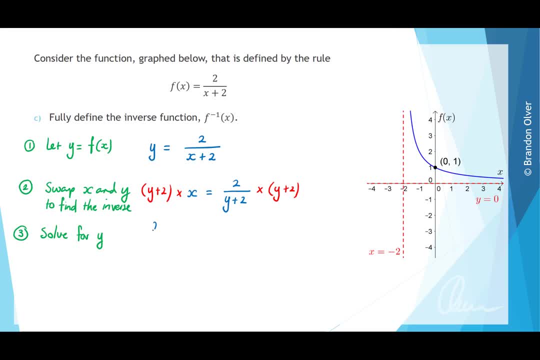 So when we do the multiplication on the left hand side, We get x, y plus 2. x is equal to 2.. And then we subtract 2- x from both sides of the equation, Which gives x- y, And then we're going to divide both sides of the equation by x to get y by itself. 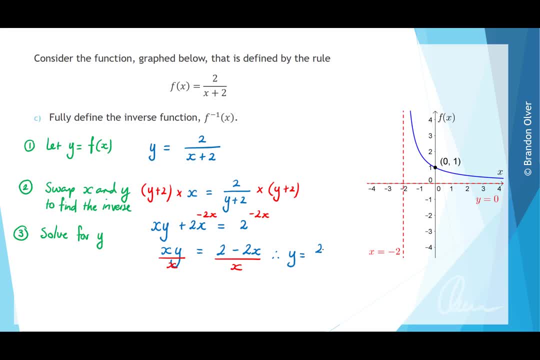 So we find that y is equal to 2 subtract 2 x divided by x. Step 4 is just to express, using the correct notation. So when we do that, we express the inverse as f. inverse of x is equal to the rule. And now this rule that we have over here can be simplified slightly. 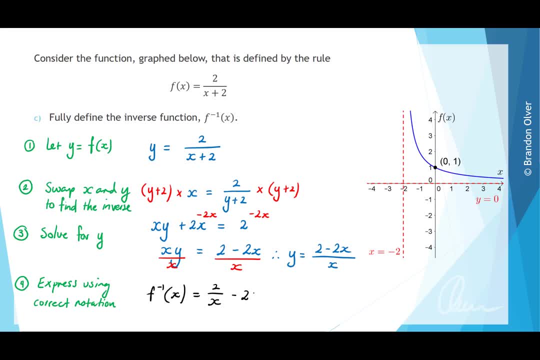 To be 2 divided by x, And then we're going to divide both sides of the equation by x, And then we're going to divide both sides of the equation by x minus 2.. And the other half of fully defining the inverse function is to state the domain. 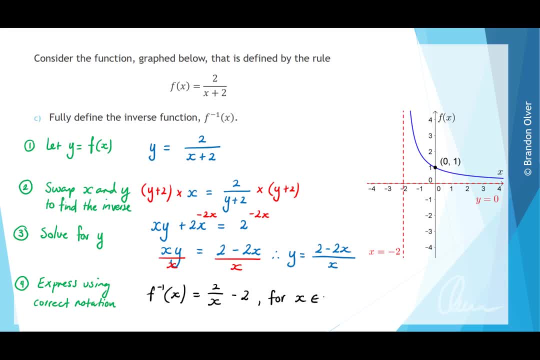 So this is going to be, for x is an element of, And the domain of this is equal to the range of the original function. So that is going to be 0 to infinity And that's what we found previously in the table in part a. 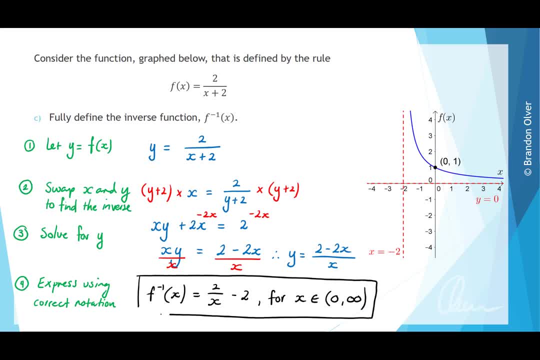 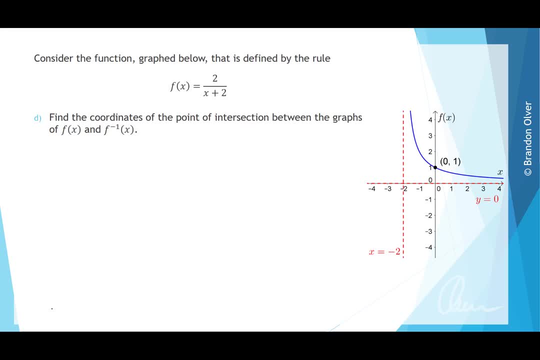 So this is the fully defined inverse function with a rule and its domain. For part d, we want to find the coordinates Of the, The point of intersection between the graphs f and f inverse, And we know that the coordinates of the point of intersection will lie along the line y equals x. 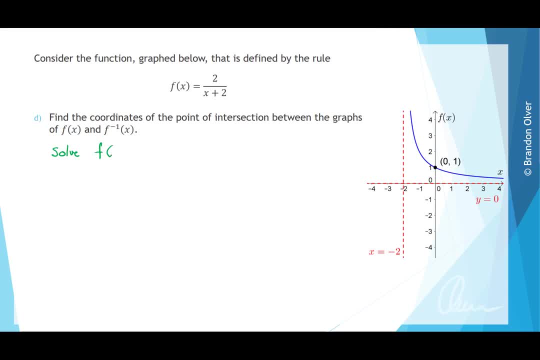 So that means we can solve f of x equaling x to find the point of intersection. So if f of x equals x, we have 2 divided by x plus 2 is equal to x. And now to solve that we want all of the variables on the same line. 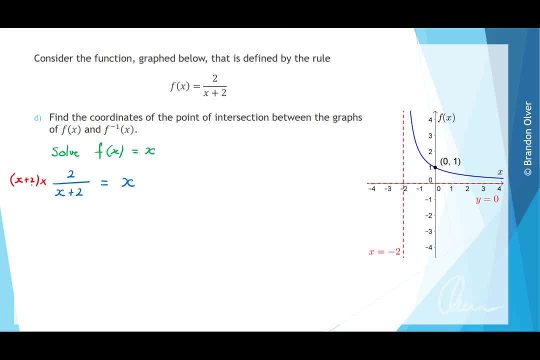 So we're going to multiply both sides By x plus 2.. And this will give us: 2 is equal to x times x plus 2.. And now to solve this, we can recognise that it's a quadratic, So we need to get all terms onto one side of the equation. 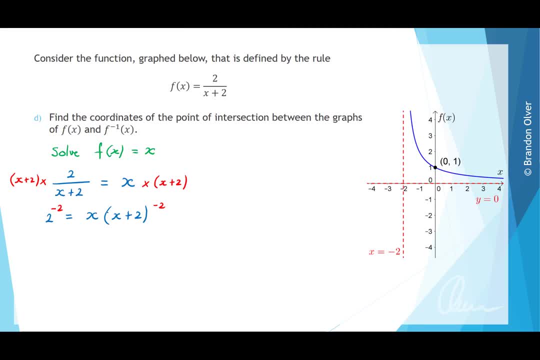 So we're going to subtract 2 from both sides of the equation And expanding the brackets will give x squared plus 2x minus 2 is equal to 0. And we can try and factorise that by inspection, but we'll find it's very difficult. 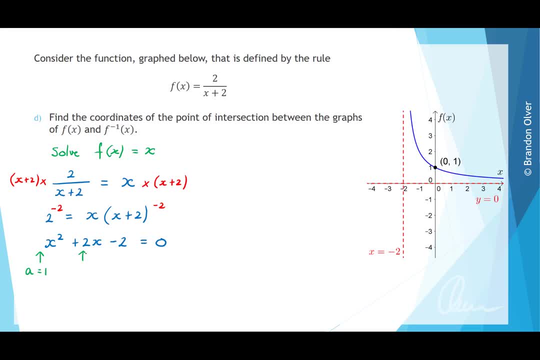 So instead We're going to say that a equals 1, b equals 2 and c equals negative 2.. And we're going to use the general quadratic formula to solve this equation. So the general quadratic formula is: x is equal to minus b, plus or minus the square root of b squared minus 4ac divided by 2a. 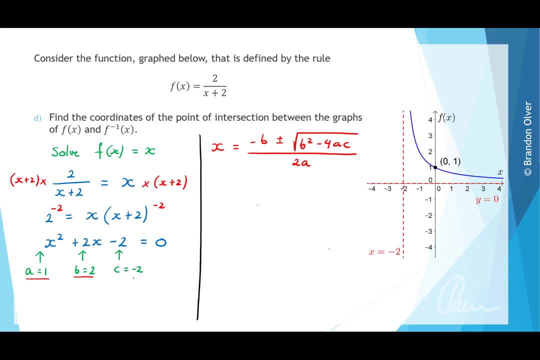 Where a, b and c are the values we found here, here and here. So if we sub those in, We find x is equal to minus b, which is minus 2, plus or minus the square root of, And we're going to have 2 squared minus 4 times a, which is 1 times c, which is minus 2, divided by 2a, which is 2 times 1.. 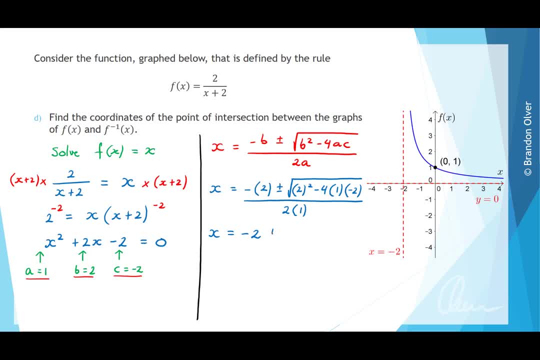 So if we simplify that, we will get: x is equal to minus 2, plus or minus. the square root of- And here we're going to have 4 plus 8 gives 12 divided by 2.. And now we know the square root of 12 can be written as the square root of 4 times the square root of 3, which equals 2 root 3.. 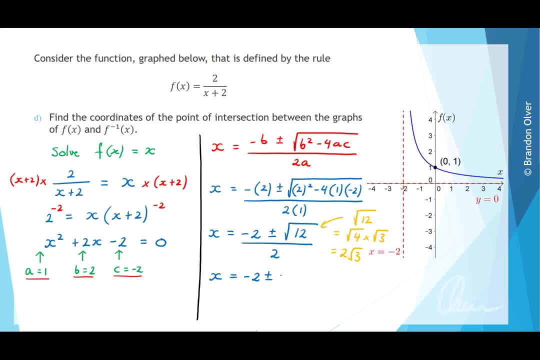 So we can write this: as x is equal to minus 2 plus or minus 2 root 3 divided by 2.. And now that will simplify down to minus 1 plus or minus the square root of 3.. However, if we inspect our domain, 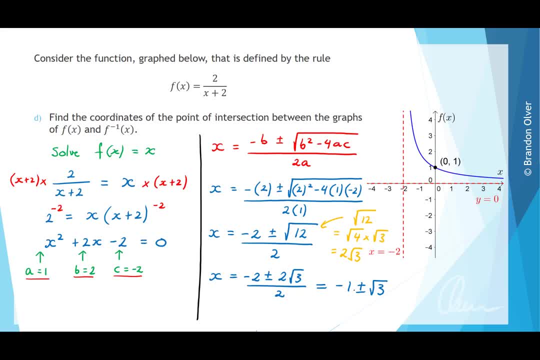 Minus 1 minus the square root of 3 is outside of the domain. So the only solution that it can be 3 is minus 1 plus the square root of 3.. And because that occurs on the line, y equals x. 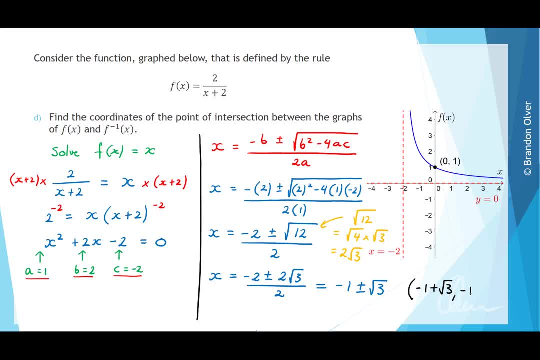 the x and y values are the same. So the y value is going to be minus 1, plus the square root of 3 also. So that is the coordinate for the point of intersection between the graph f and its inverse. So for part e, on the same set of axes as the function f, we 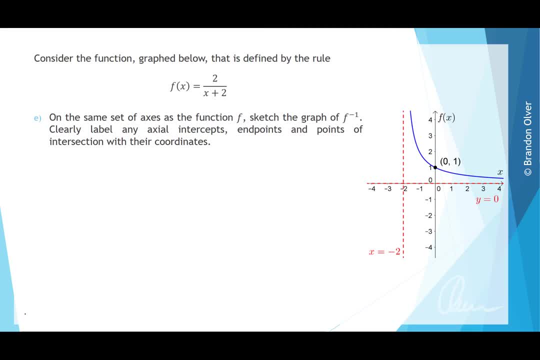 want to sketch the graph of the inverse And we want to clearly label any axial intercepts, endpoints and points of intersection with their coordinates. Previously we found that f inverse of x was equal to 2 divided by x minus 2, for x is an element of 0 to infinity. 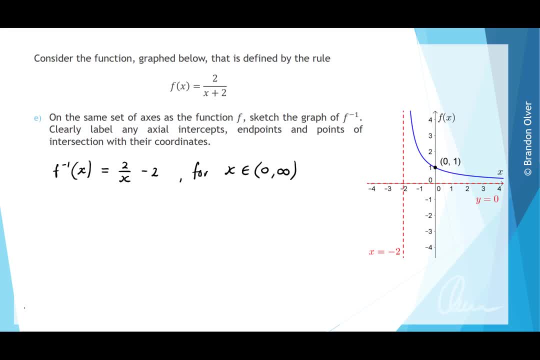 So that is the part of the graph that we need to sketch. So, because x and y have been swapped, we now have our vertical asymptote, which I'm drawing in here with the red dotted line: is going to occur at: x equals 1 plus the square root of 3 plus the square root of 3.. So that is the part of the graph that we need to sketch. So, because x and y have been swapped, we now have our next intercept. So we have the x intercept of 0 plus x minus 3 plus x minus 2 plus the square root of 3 plus the square root of 3.. And we can think of this as the 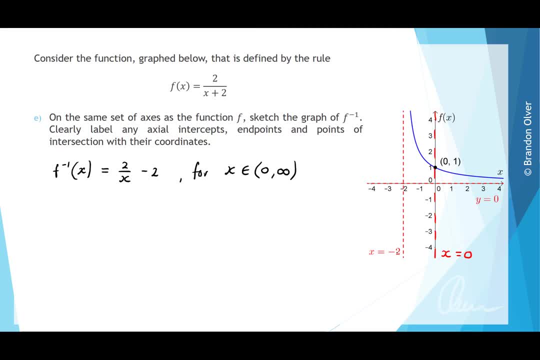 full-term relationship. So in this example we have an x intercept of 0 to infinity. at x equals 0, where it was previously y equals 0 and where x was previously negative 2, we now have y is equal to minus 2 as the other asymptote. 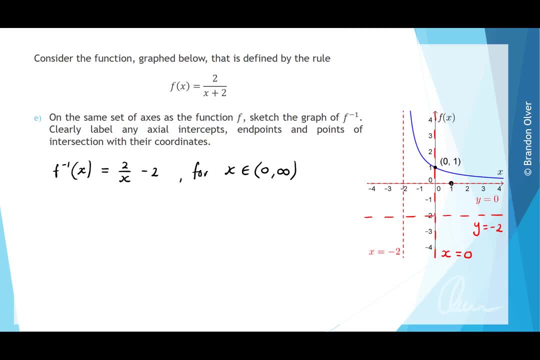 The y intercept of 0, 1 now becomes an x intercept of 1 comma 0.. Sketching the inverse hyperbola through these points gives this curve here, And the last thing we need to do is sketch the intersection of f and f inverse, which. 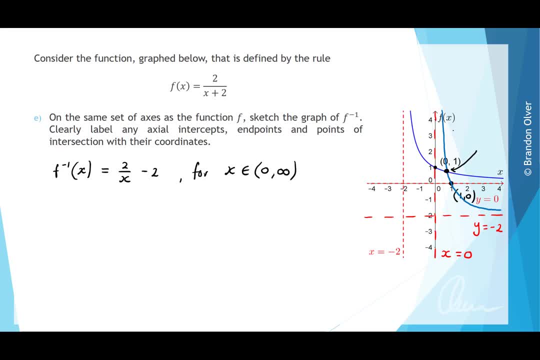 occurs at this point here And in part d we found the coordinate there was minus 1 plus root 3, comma: minus 1 plus root 3.. So that is the coordinate of the point of intersection for the graph. So this graph here is f inverse of x.